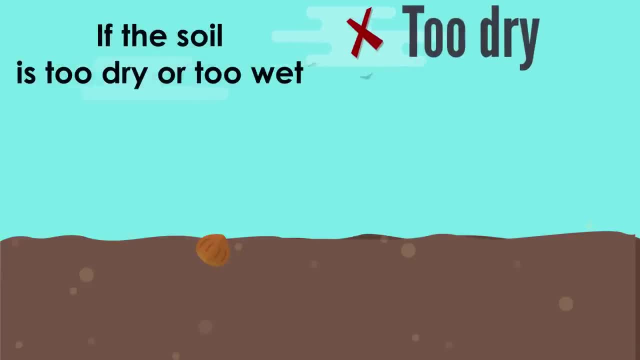 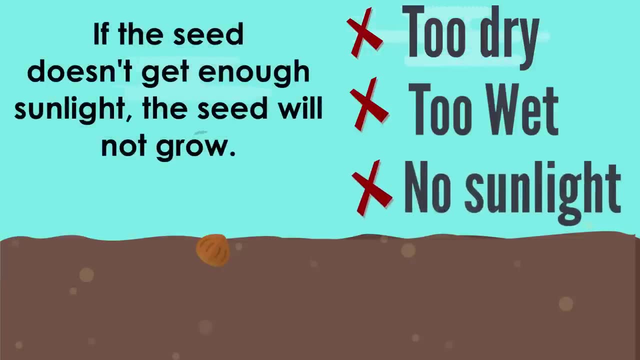 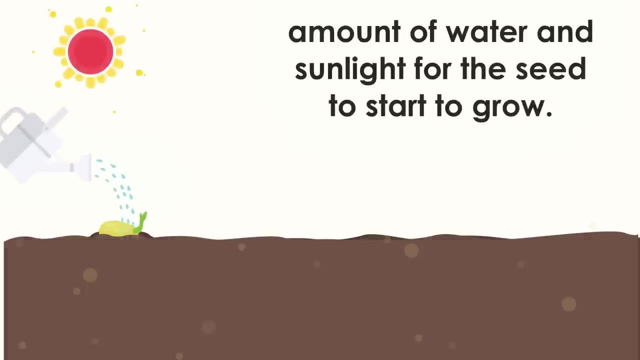 If the soil is too dry or too wet, the seed might not grow. If the seed doesn't get enough sunlight, the seed will not grow. The seed needs to get a root. It needs the right amount of water and sunlight for the seed to start to grow. 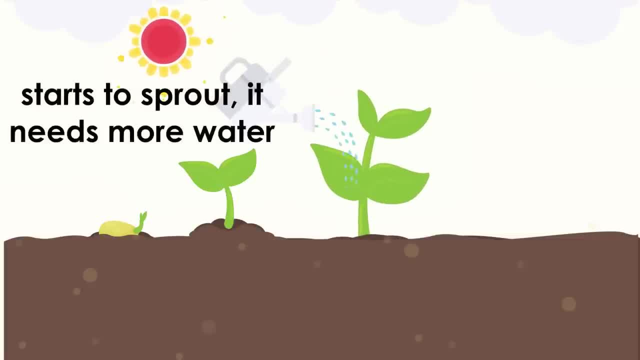 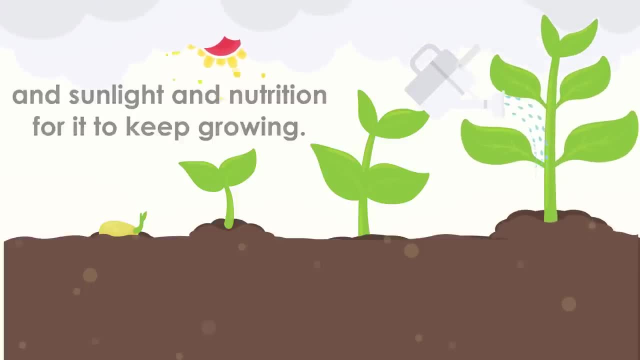 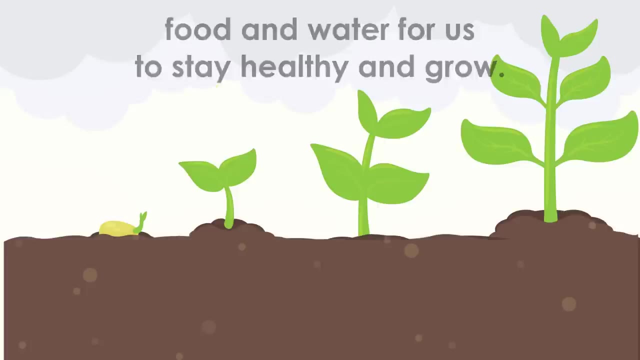 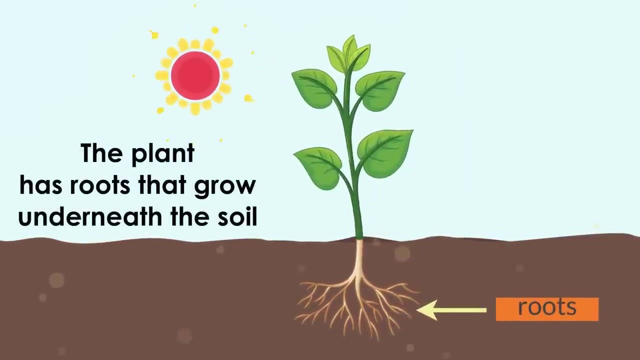 Then, once the seed starts to sprout, it needs more water and sunlight and nutrition for it to keep growing, Just like you and me need nutrition from food and water for us to stay healthy and grow. that's what plants need. The plant has roots that grow underneath the soil. 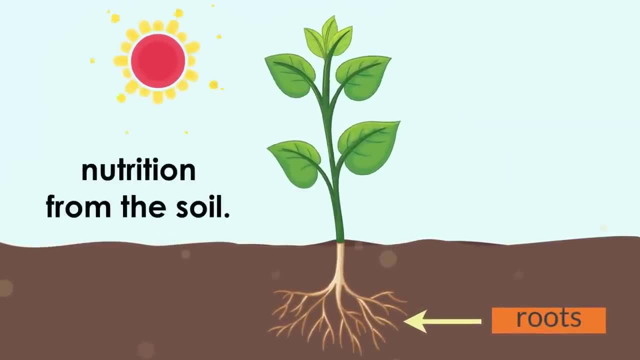 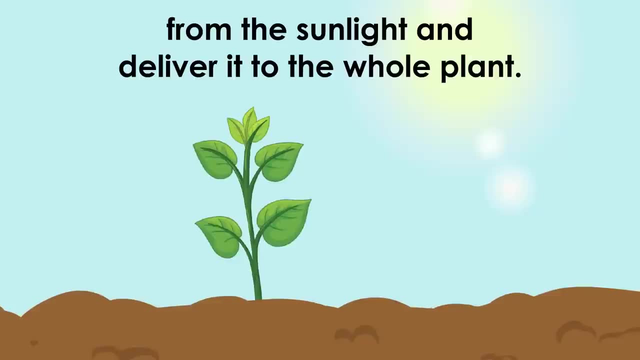 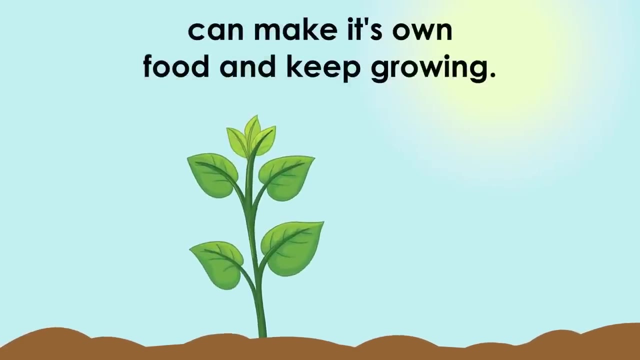 And that is where it collects water and nutrition: from the soil. The leaves get energy from the sunlight and deliver it to the whole plant. With all those ingredients, the plant can make its own food and keep growing To help the plant grow faster. 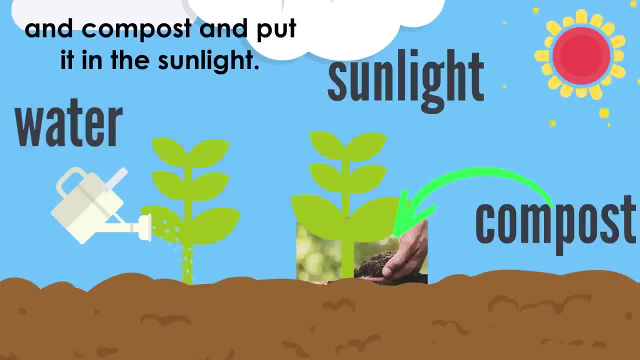 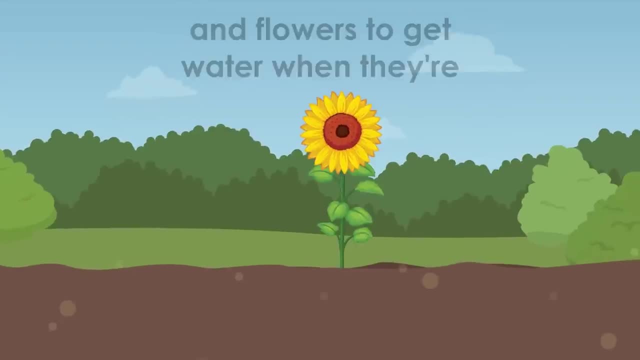 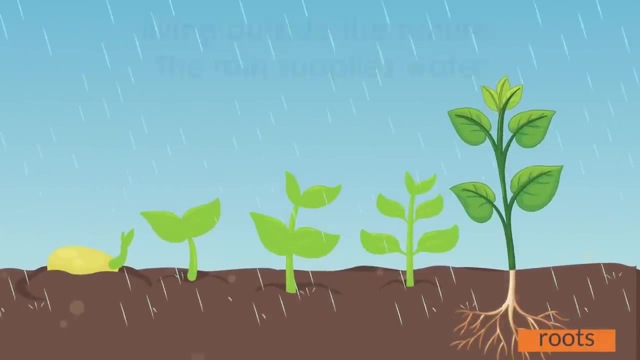 we give it water and compost and put it in the sunlight. Rain is the perfect way for plants and trees and flowers to get water when they are living outside in nature. The rain supplies water to the soil and the plant drinks it up in the roots. 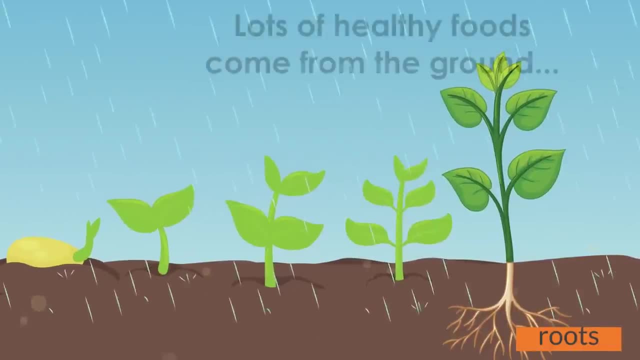 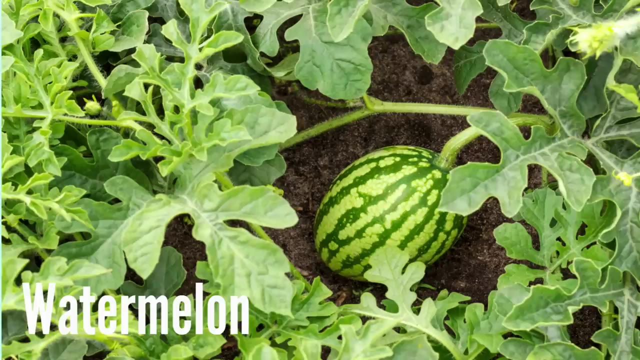 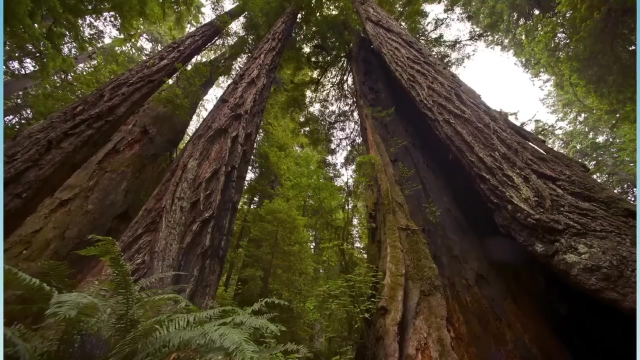 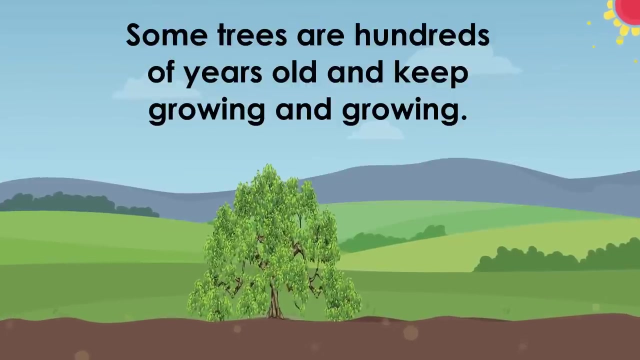 And that helps the plant grow. Lots of healthy foods come from the ground: Carrots, lettuce, potatoes, watermelons. What food can you think of that comes from the ground? Have you ever looked at a huge redwood tree? Some trees are hundreds of years old and keep growing and growing. 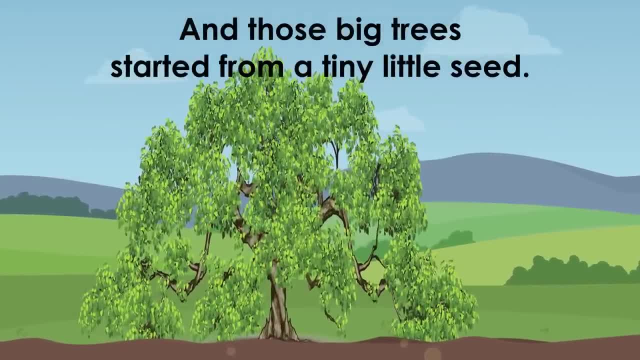 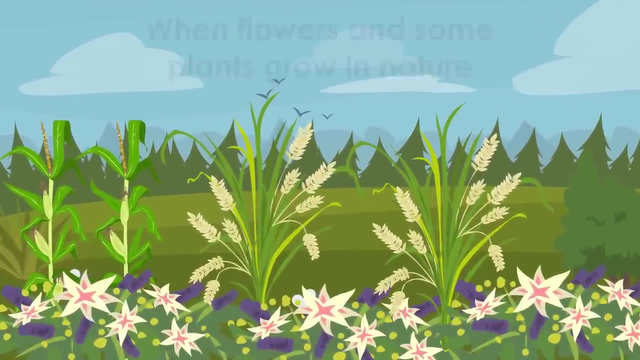 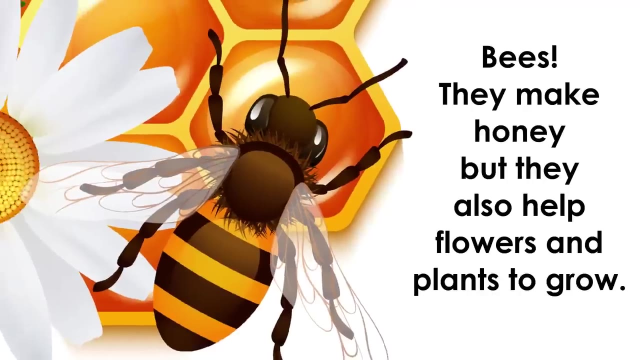 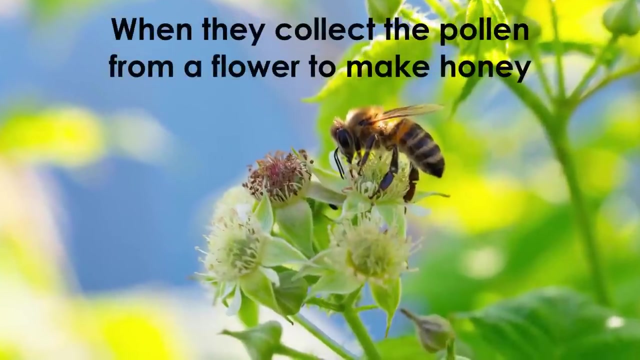 And those big trees started from a tiny little seed. When flowers and some plants grow in nature, do you know what helps spread their seeds all over Bees? They make honey, but they also help flowers and plants to grow When they collect the pollen from a flower to make honey.